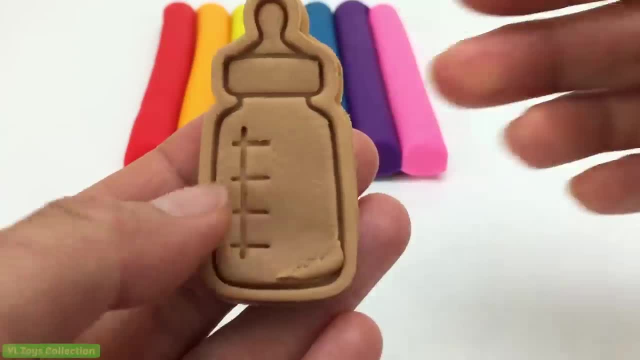 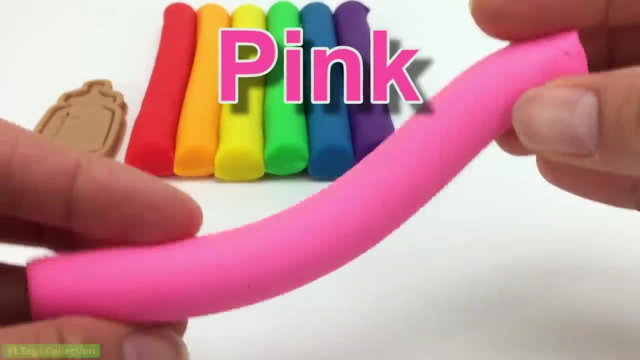 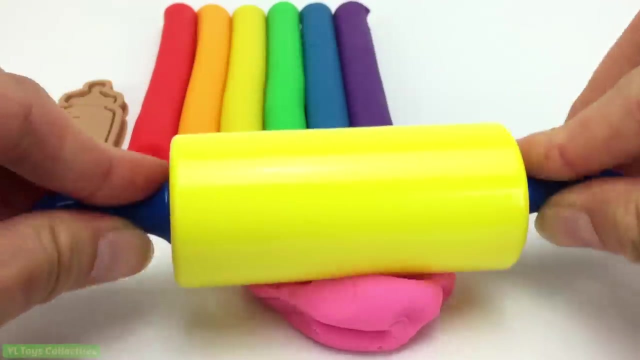 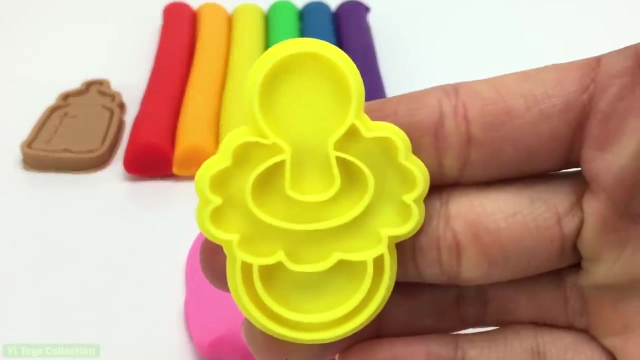 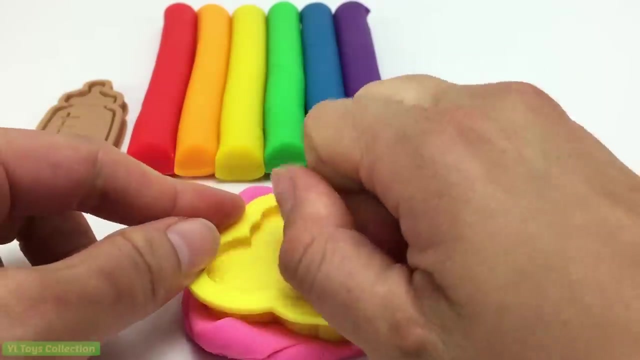 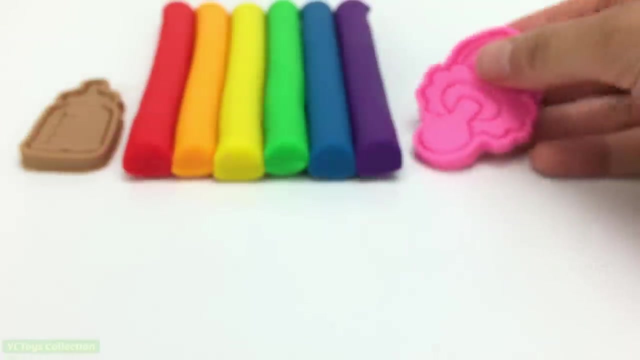 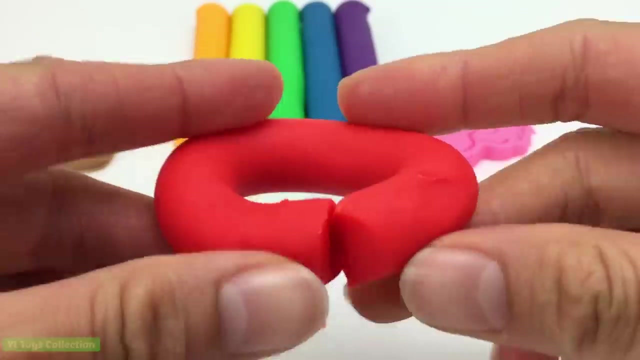 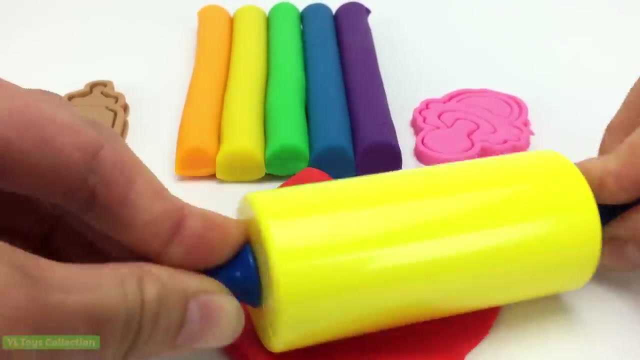 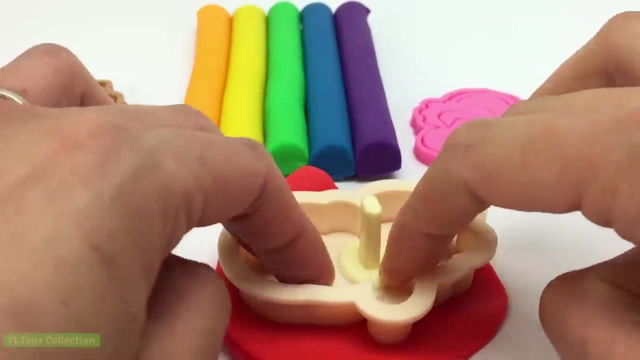 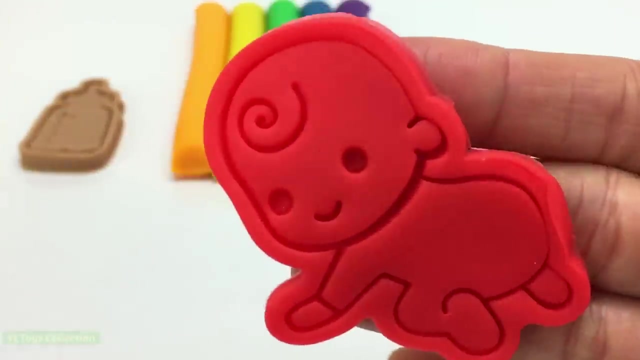 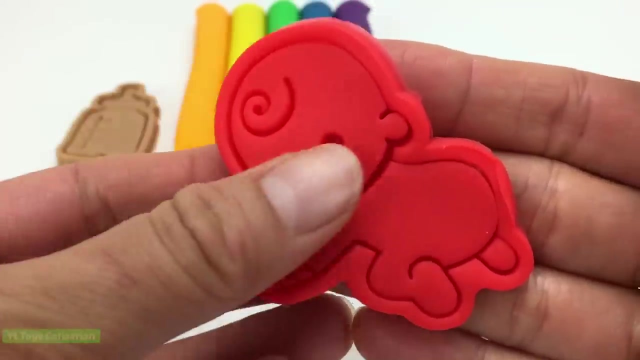 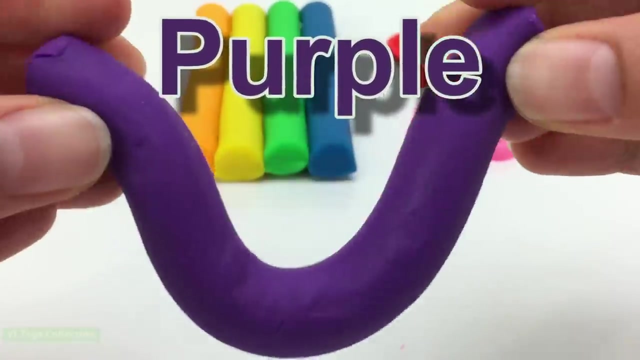 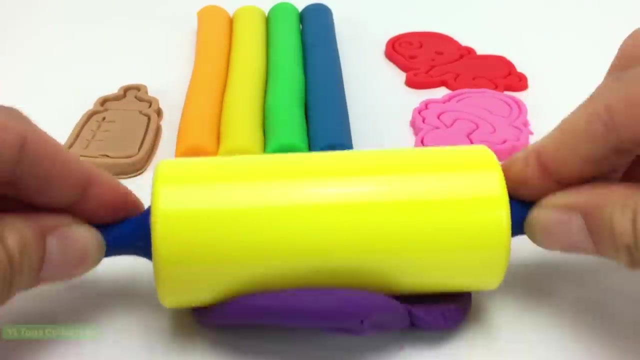 37,, 38,, 39,, 40, 30,, 40,, 41,, 42,, 43,, 5,, 6,, 7,, 8,, 8,, 9,, 10. Oh, Pink, Red, Purple Orange. 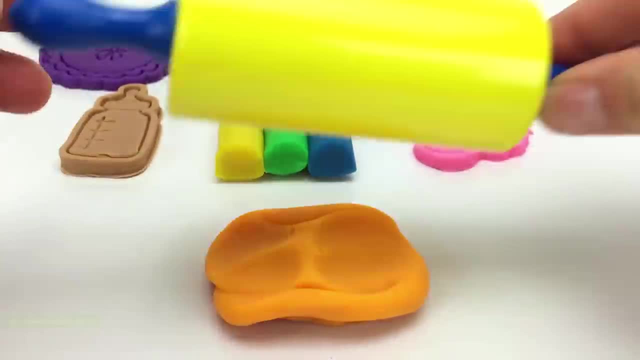 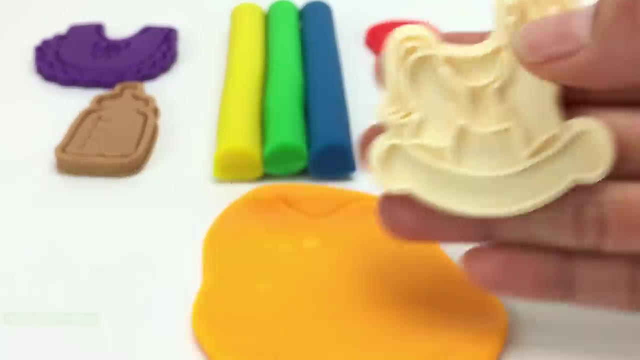 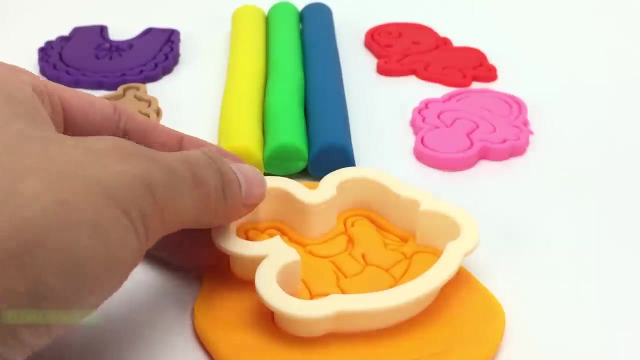 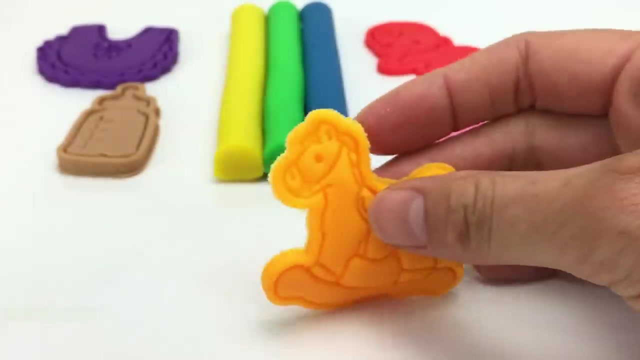 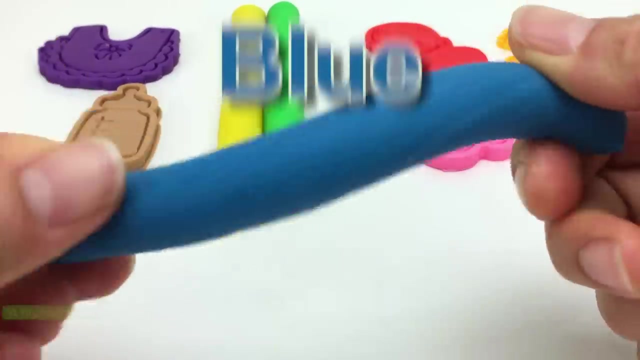 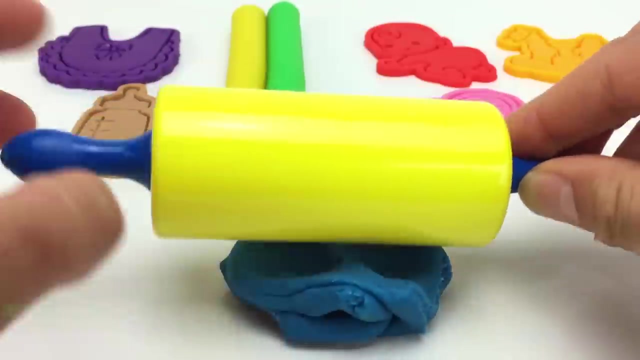 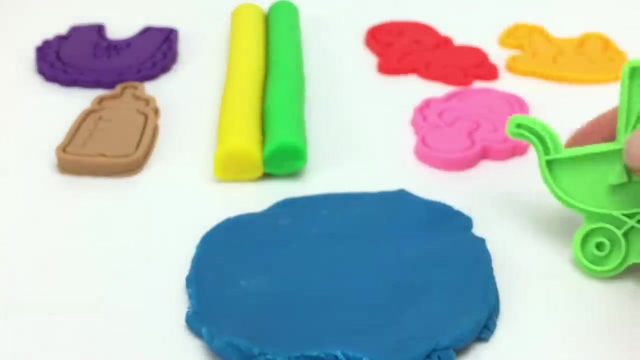 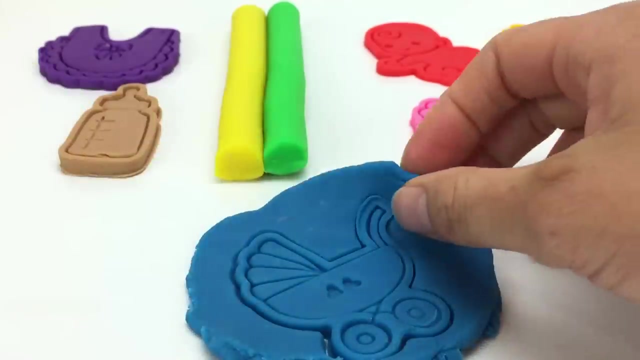 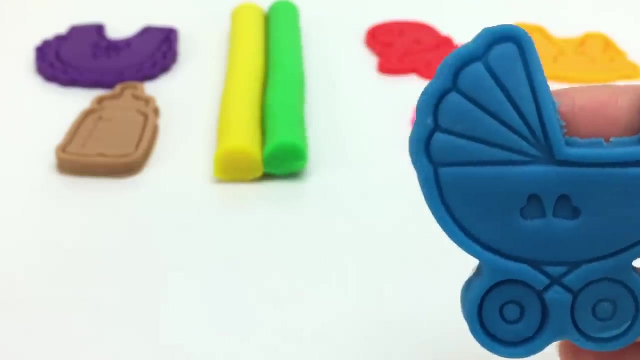 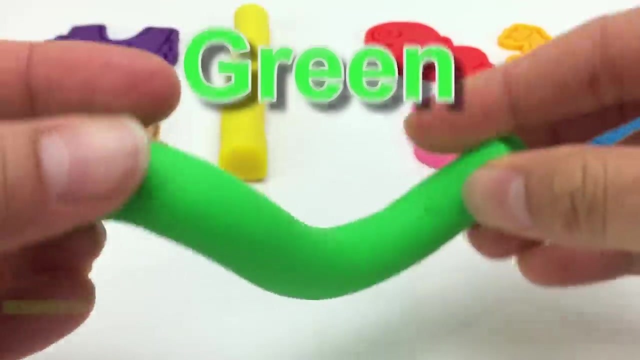 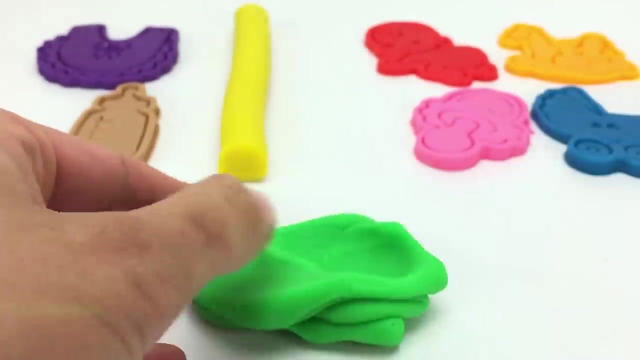 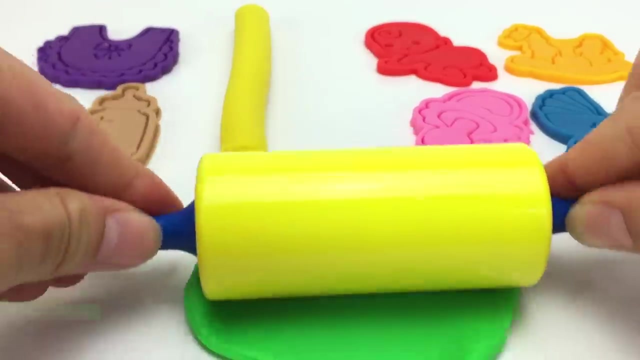 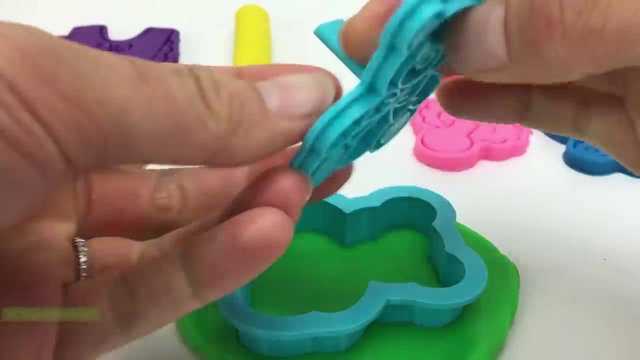 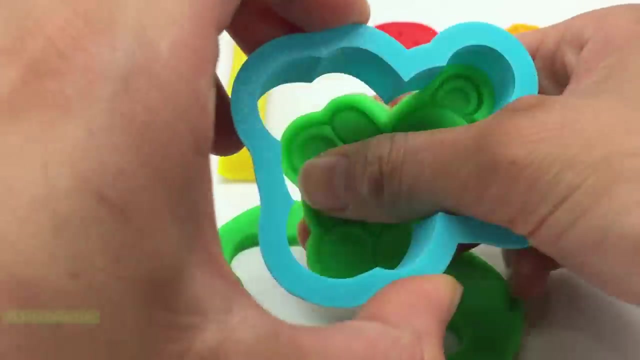 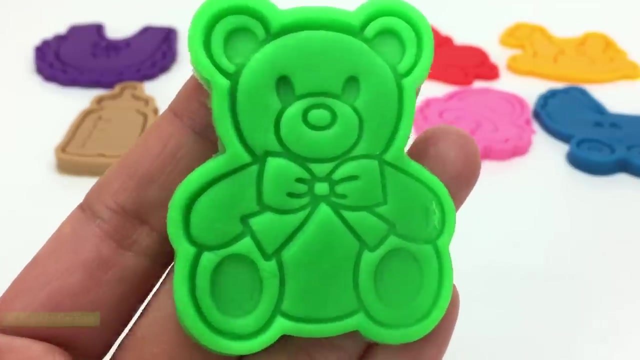 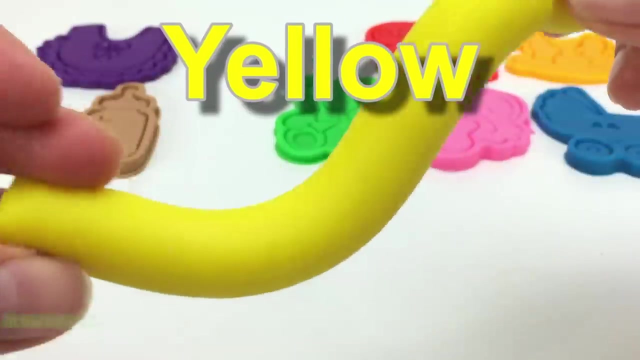 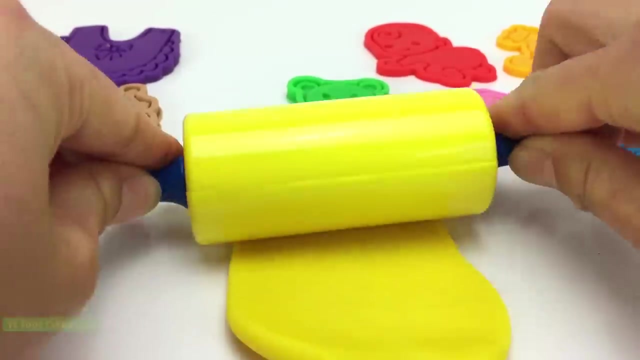 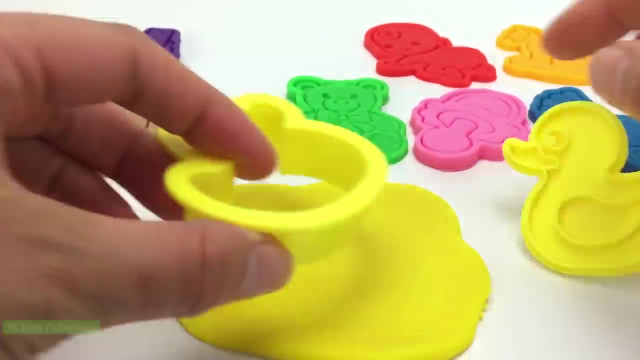 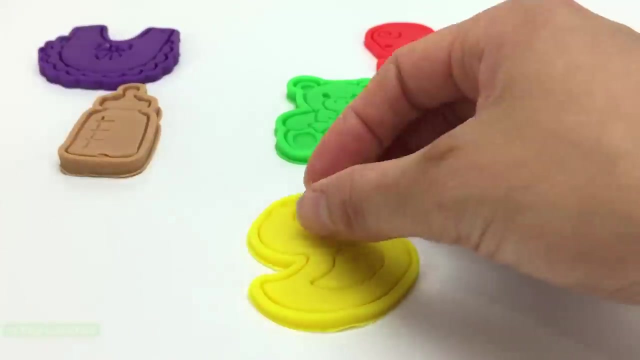 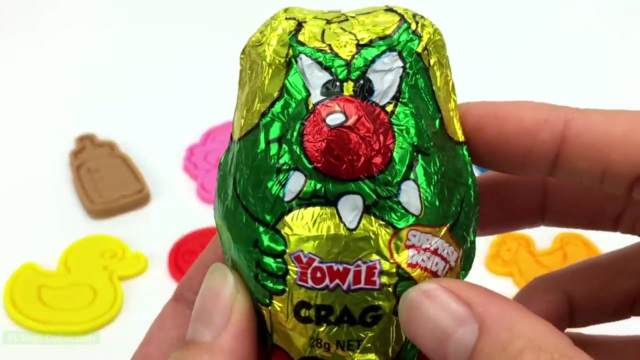 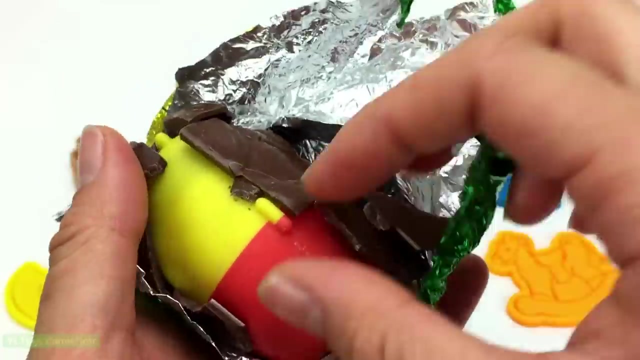 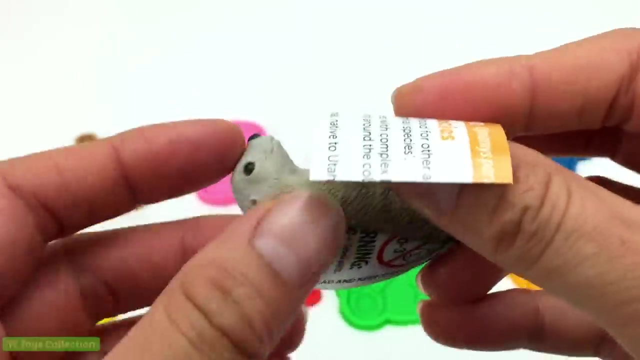 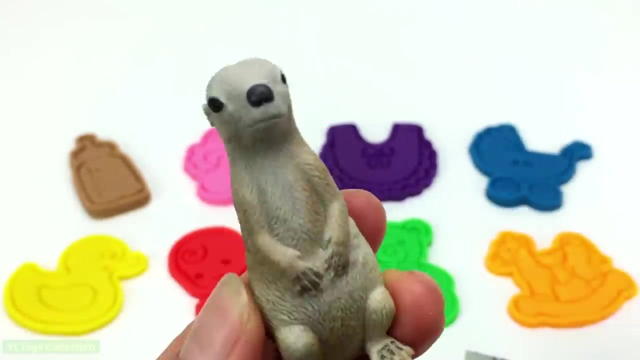 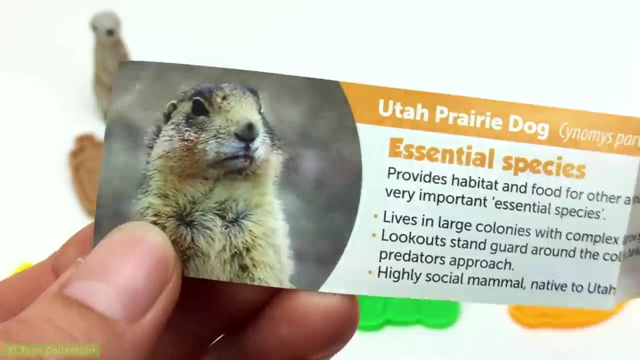 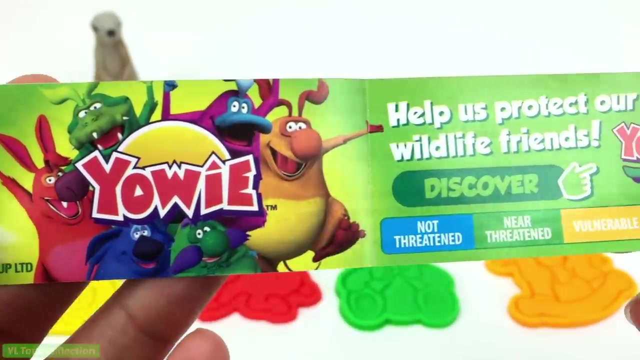 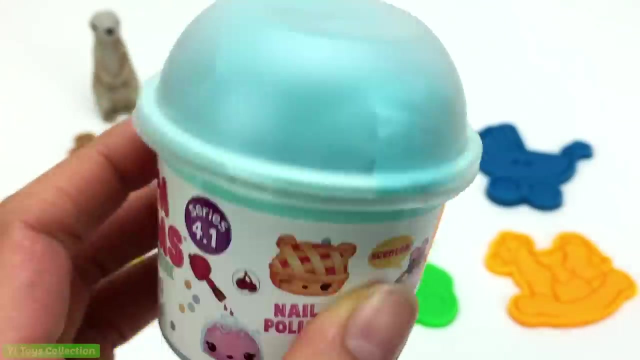 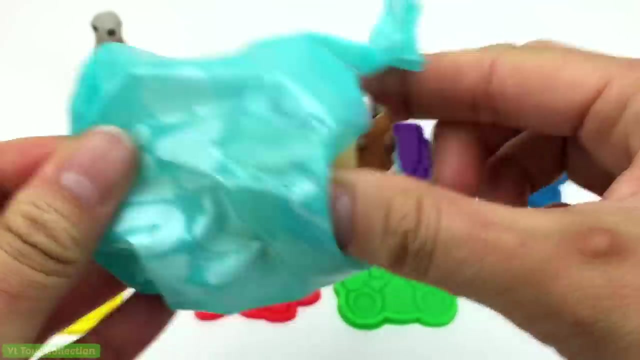 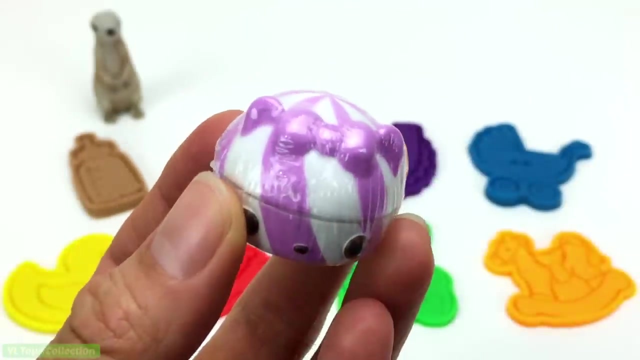 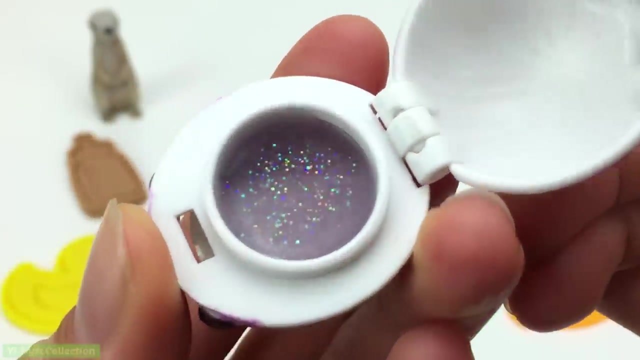 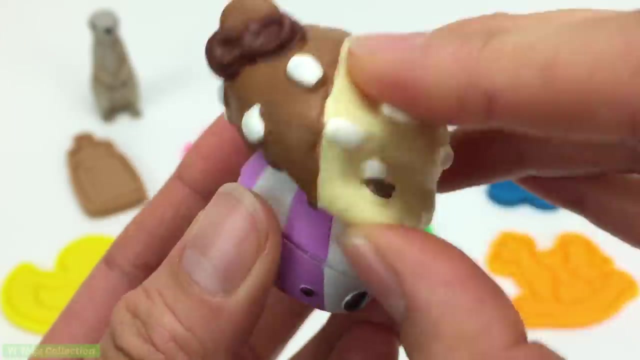 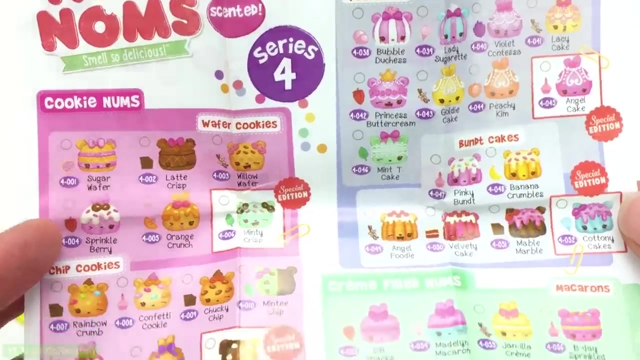 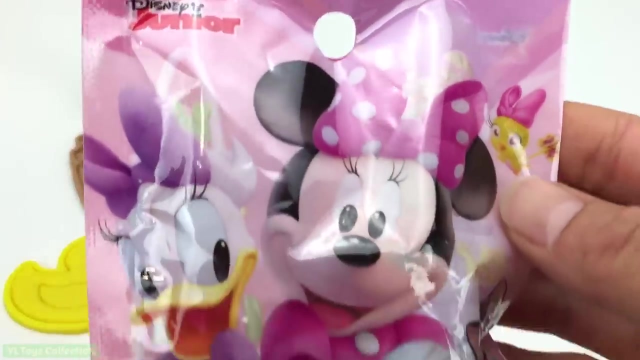 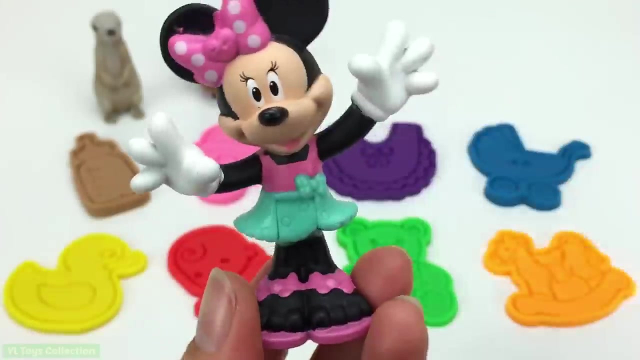 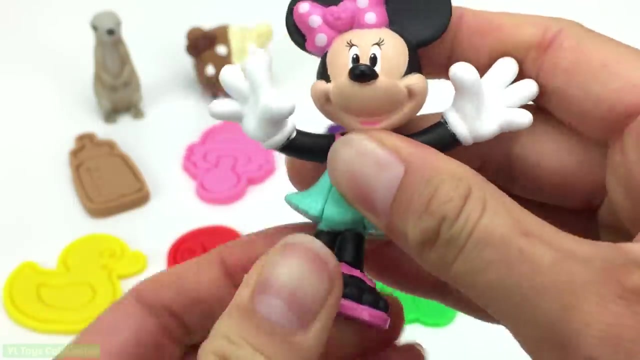 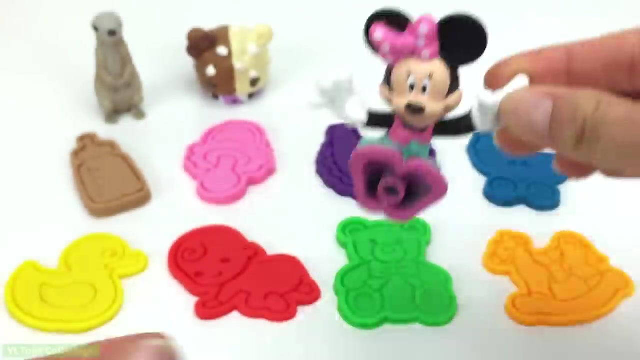